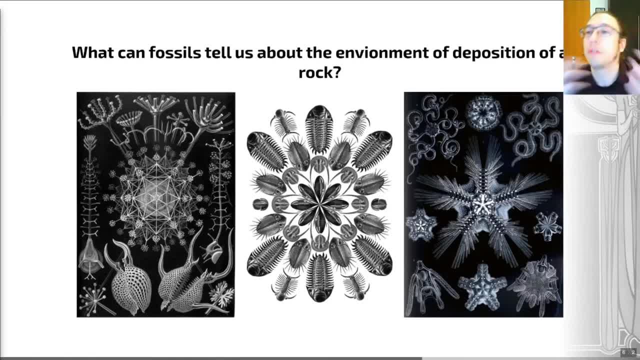 the changes and conditions that we're going through, and the changes in the history of life and the changes in the life system. conditions are a key part of that equation, and so using fossils in this way can help us untangle some really complicated pictures, if we have enough data when we're looking. 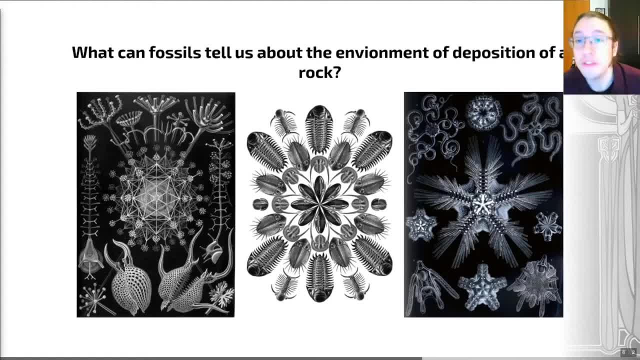 at the fossil record. So a key takeaway message from this video is that, as well as telling us about past ecosystems and life, paleoecology is important because it can tell us about rocks and the depositional history of that rock. If you're coming from a biology background, 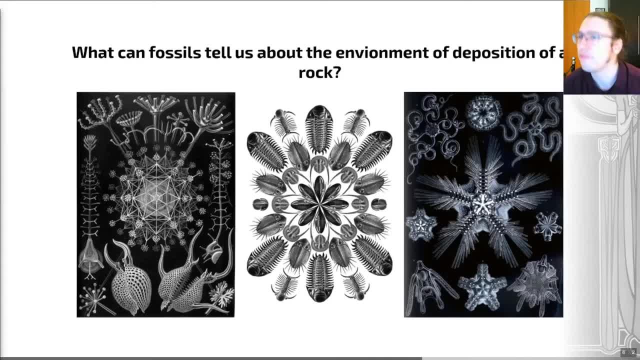 I wanted to highlight that because that may not be obvious, but that is, in fact, a really useful thing that fossils can help us with. The geologists amongst you may be sitting there nodding along, going like yeah or not, as the case may be, So for the geologists, 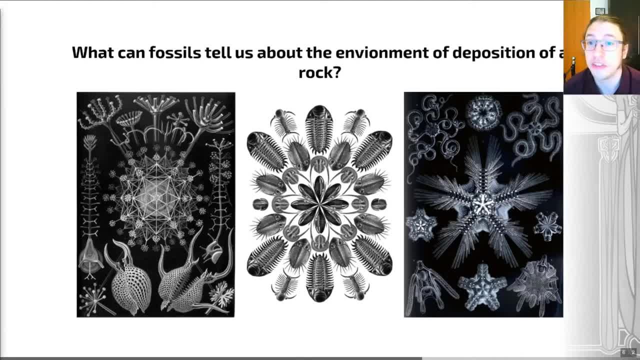 amongst you, you will probably be familiar with the idea that sedimentary information is key when it comes to evidence for the environment of deposition of a rock in many circumstances. For those of you that haven't done geology before, that will include, for example, the grain size of a sedimentary rock That can tell you about the energy. 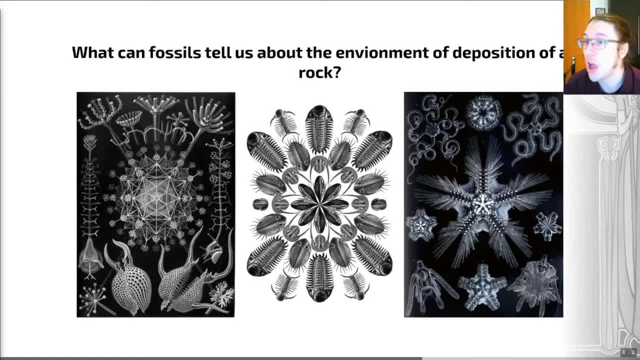 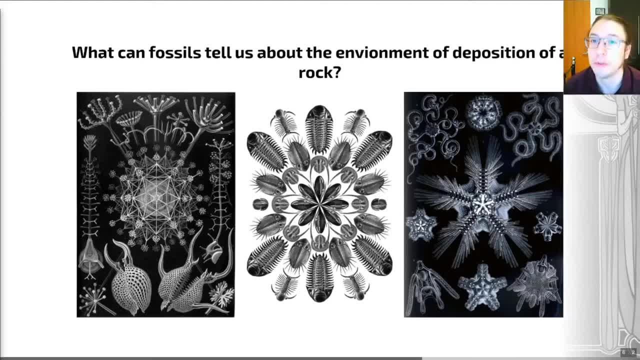 can carry larger grains than small energy, water, for example. But fossils can aid that interpretation. They can tell you what was going on because they depend upon the environment, because ecological niches and interact with environmental gradients. So this is something that's complementary to the world of sedimentary geology. 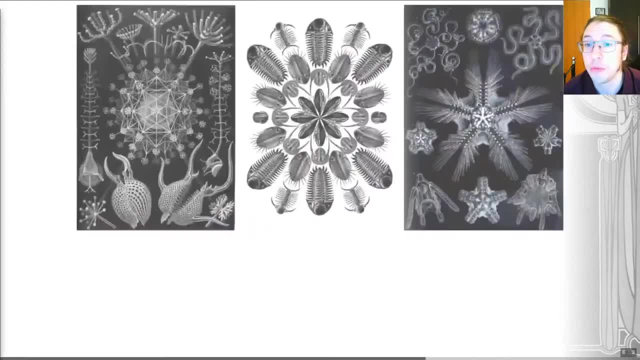 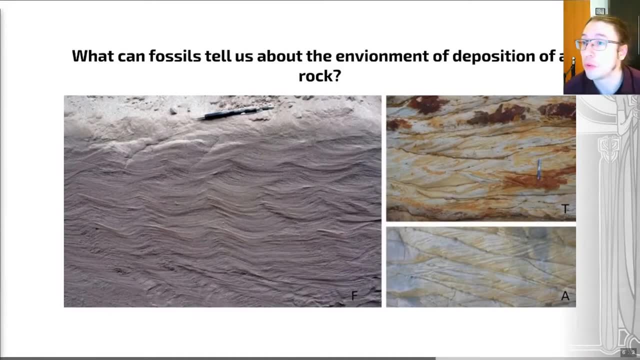 And between them the sediments and fossils, can help us build a very clear picture of picture, but sometimes fossils alone are really integral. these are examples of what are called cross stratified sandstones. yeah, so this structure here is cross stratification. for those of you that have never done geology before this: 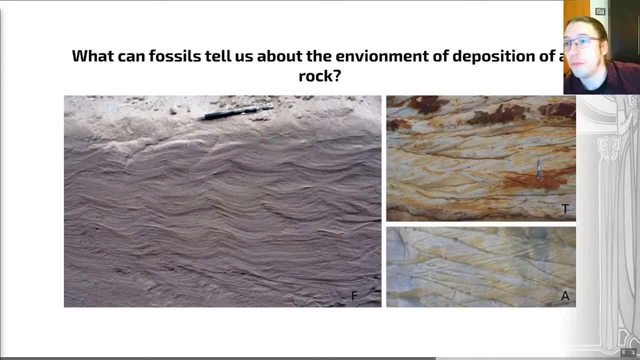 just means that our rock was deposited under some kind of flow of some kind of fluid, be that water or air, and indeed in cross stratified sandstone such as this, it is impossible to tell from the rock alone whether the rock was deposited in a fluvial, so a river based environment such as this example here, whether it was. 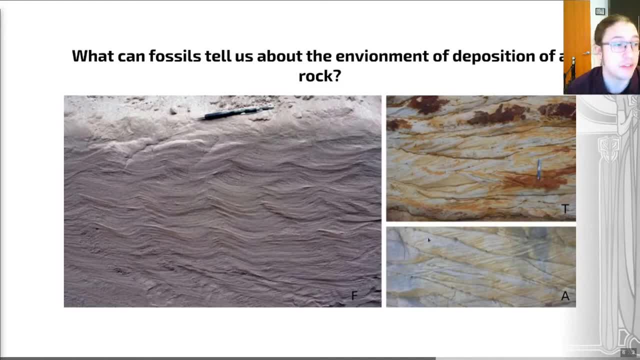 deposited in an aeolian environment, so a desert. that's this example here. or whether it was deposited in, say, a tidal environment- that's this example here. the fossils can do that and it's in its simplest form. if we find a marine bivalve in a bit of rock, we know that it wasn't deposited in a fluvial or a aeolian. 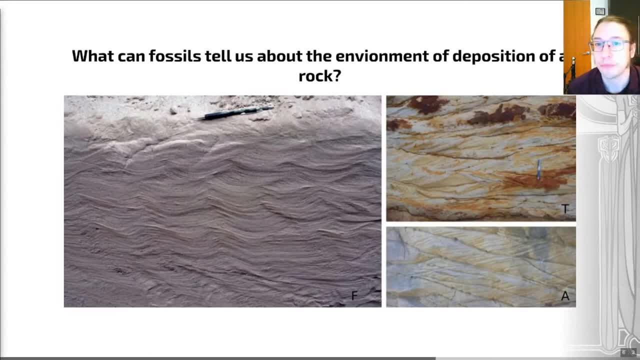 environment, so it must be tidal. up here, if we find a freshwater organism, well, it certainly can't be a desert and it's probably not tidal, because then you have too much salt in your water. therefore, we're looking at a fluvial environment as an example for the geologists amongst you. mudstones are 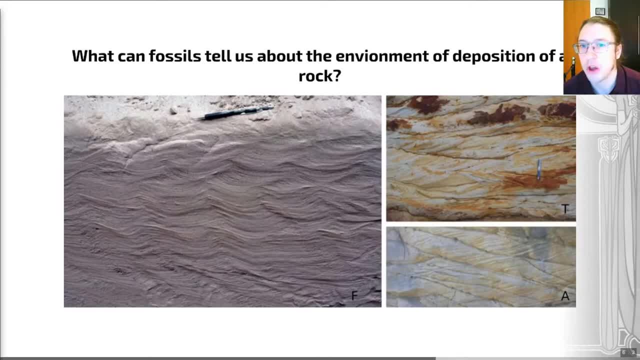 notorious for providing very little information. it's very hard to tell an oceanic deposit from a river flood from a deep marine sediment, and fossils can also tell you about things like the firmness of the substrate, the rates of sedimentation of a rock, your paleo latitude and your paleo climate. so 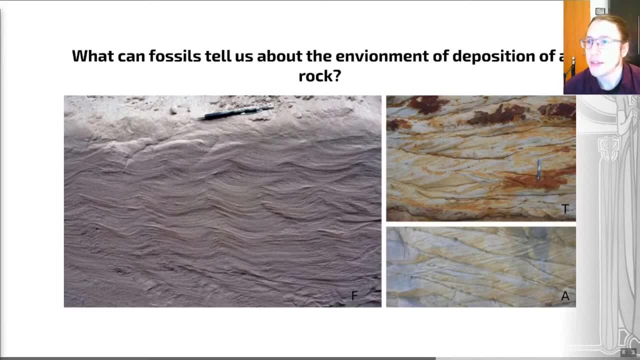 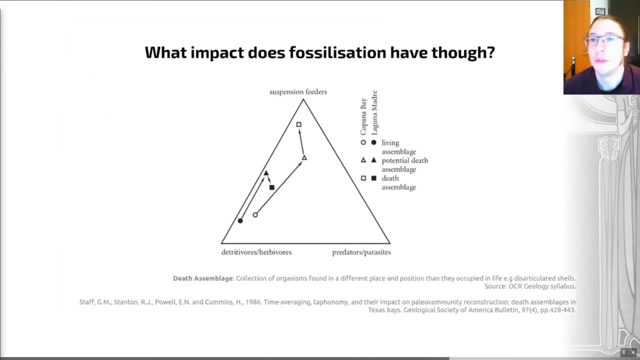 they're really, really useful. so that is hopefully matching, getting us all on the same page, no matter where we're coming from, be we biologists or geologists. fossils in rocks can be really, really useful, but we've got to consider the impact that the process of fossilization 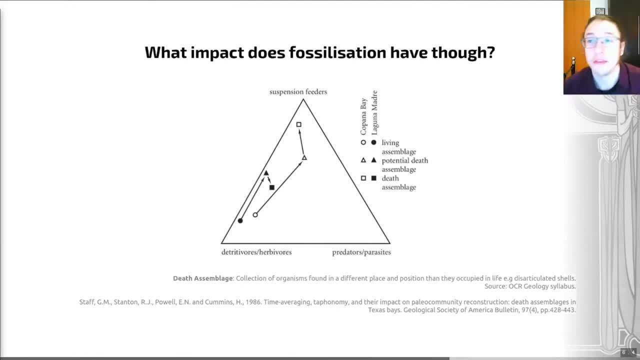 actually has. this is a thing that's called tofonomy, and this is a topic that Rob will be covering later in this course. you'll have another one more lecture from Rob covering the topic of tofonomy, but we have to consider this when we're speculating about environments, so biases exist in. 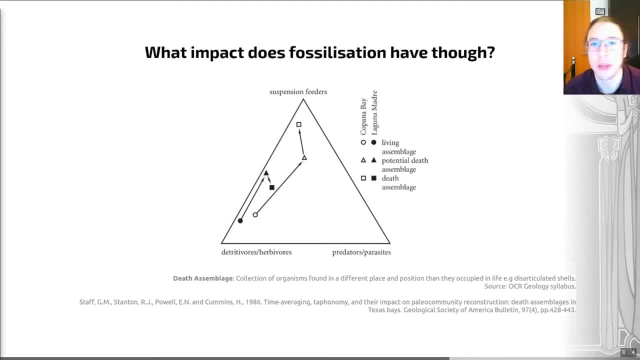 fossilization, and this will be a key part of your tofonomy lecture. hard parts preserve and soft parts don't. that's the long list of things we're going to be talking about in the next lecture. so we have a thing, an idea within paleontology, called the death. 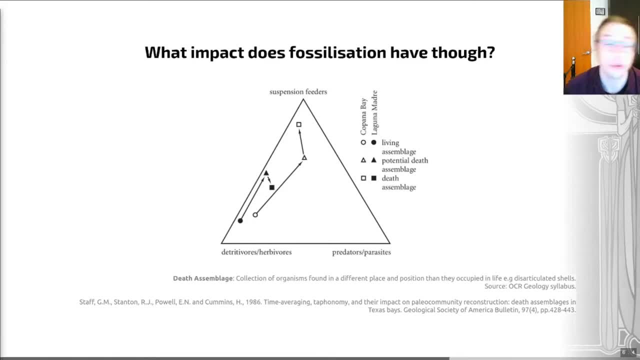 assemblage. this I've defined on the slide for you here. this is the collection of organisms found in different place and position to that which they occupied in life. this would be the disarticulated shells. this reflects that after an organism dies, it is often moved around. you have different 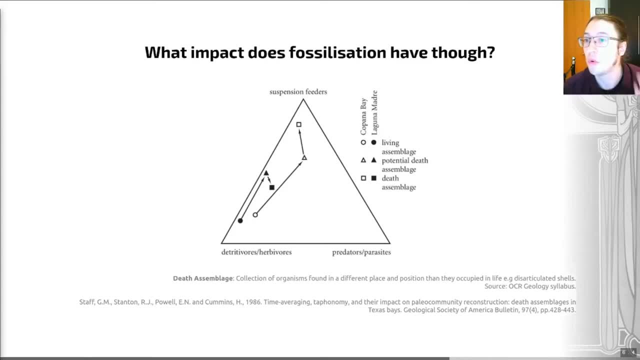 changes occur to the remains of the victims of the death and the death of the of these organisms before they're deposited in the rock, And we can assess the similarity of a death assemblage to its living counterpart in different ways. This we may refer to as the fidelity. 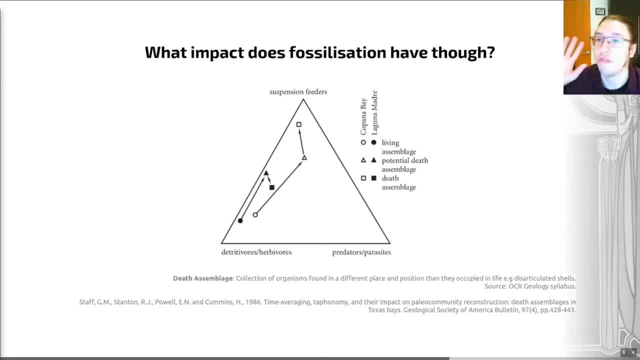 of that death assemblage, how much it represents what was originally alive. There are relatively few studies on this particular area, though I note that one actually came out today. I'm recording this- at the end of October, and there's a paper that was released. 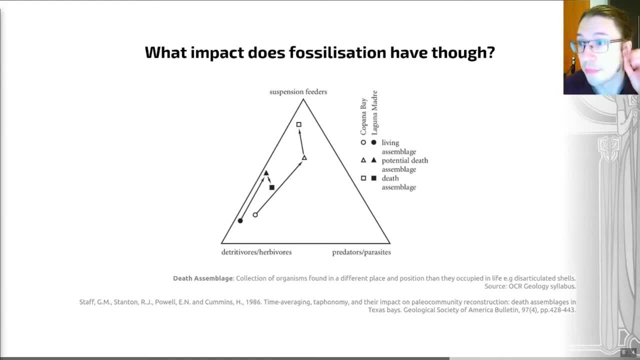 about half an hour ago that was actually looking at fossilization biases in the marine realm, which I'm really excited to read, but came a bit too late for me to include in this lecture, so bear in mind that. So the example that I've chosen instead. 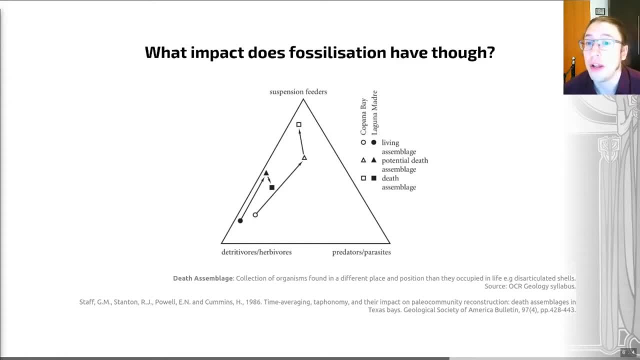 is a series of detailed studies on living and dead faunas of a place called Copana Bay and the Laguna Madre along the Texas coast. This is the paper. It's by George Staff et al in 1986.. So this guy, George Staff, and his colleagues. 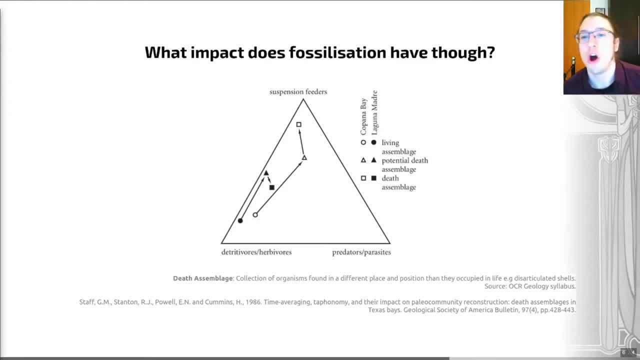 probed the paleoecological significance of the taphonomy of a number of different nearshore communities, sampled over numerous years, And what they showed is that most animals living in communities are not usually preserved. That shouldn't be a major surprise to us. 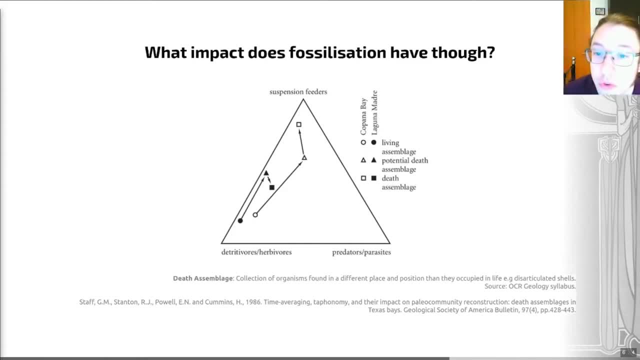 We know that only those animals that make hard parts tend to make it through to the fossil record. Nevertheless, they reported that the majority of animals with preservation potential, ie those organisms which were shelled and so were likely to be preserved, are in fact fossilized. 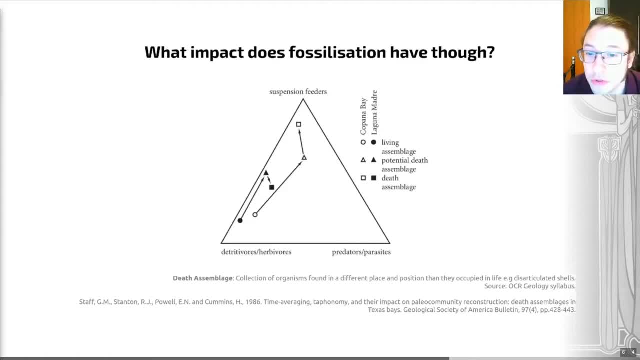 Most fossils were found in death assemblages, So most of them represent some form of post-mortem transport and some kind of mixing up of these fossils rather than being found in their life position, And this means that the effects of time averaging on what we are seeing were quite significant. 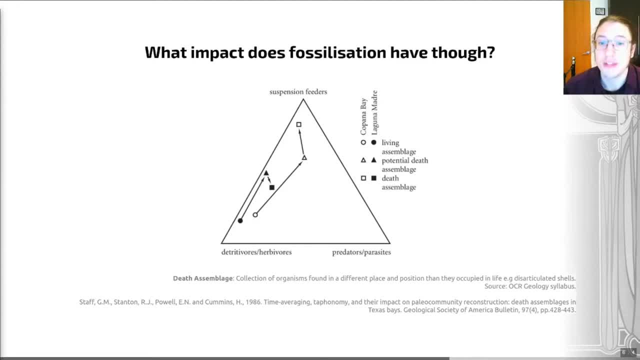 Those shelled organisms that survive through to the fossil record tend to be suspension feeders and infernal organisms, those living in sediment. Those are the most likely to be preserved and that actually modifies the paleoecological signal we see in the fossil record. 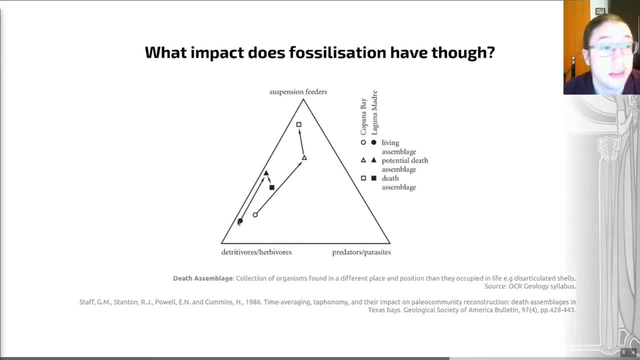 And you can see that very clearly in these two deposits on this diagram. Here we have the living assemblages which are dominated by detritivores, in this particular instance Through the taphonomic fossilization process. in both of these examples we move far further towards. 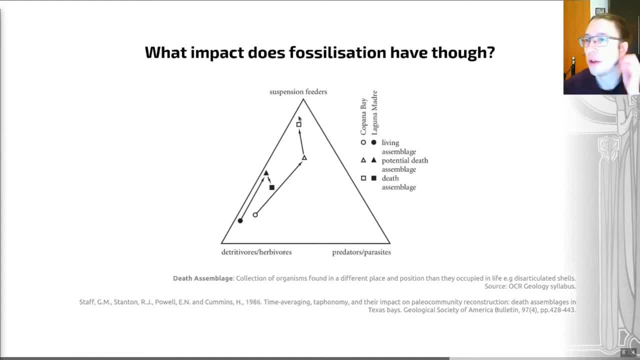 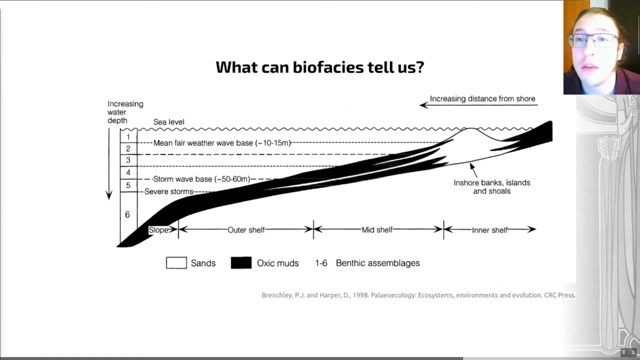 having a high proportion of suspension feeders within our ecosystems. So this is something of which we should always be aware when we're thinking about ecologies and sin ecology in the fossil record. Despite this element of bias that creeps in, you can use fossil assemblages to tell you the likely environment. 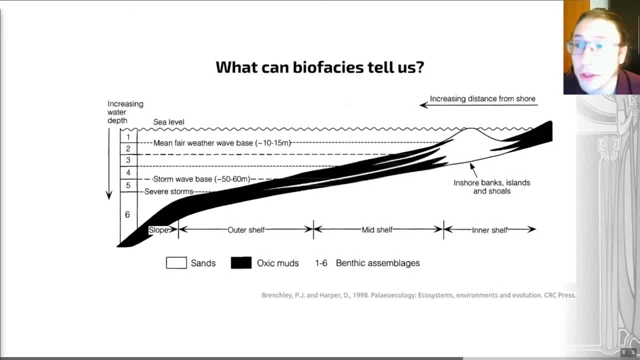 in which a rock was deposited. So I wanted to give you an example of that, and the example I've chosen is a thing called a clastic shelf. This is the kind of the bog, standard, typical sedimentary environment that you get from a sandy beach as you get increasingly deeper in the ocean, towards the, towards the. 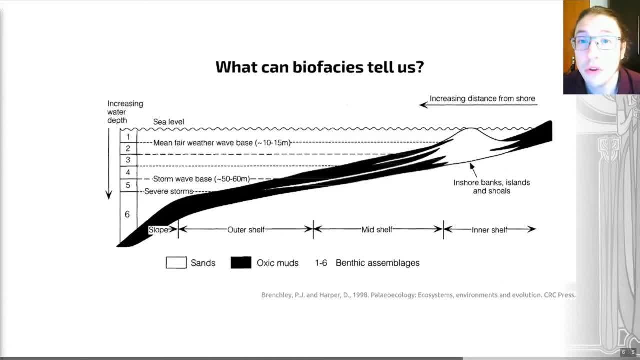 deepest parts of the ocean And you can split that kind of shelf into a number of zones, from shallow to deep, based on the fauna that's present there, that is present there and thus the fossils that we find in rocks deposited at those water depths. and this works because the composition changes with 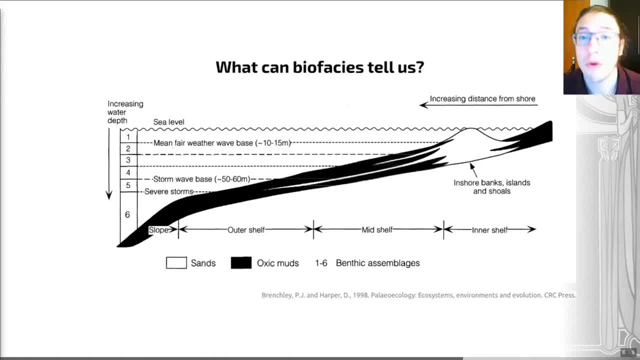 environmental gradients. There are a number of broadly defined groups or collections of organisms that we would call biophasies or benthic assemblages. In particular, WorkToDate has identified six benthic assemblages, which are based on both the lithologies, the toponomy of the fossils, the invertebrate. 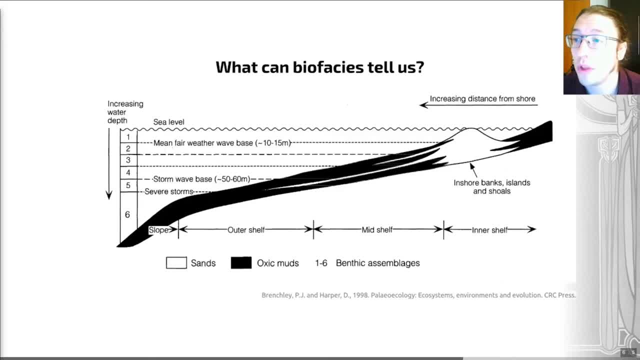 fossils that you find in these rocks and, as well as that, the trace fossils that you tend to find in these different water depths, And this diagram here shows how those zones map to the depth of water for continental shelf. Now, understanding sea level change is essential for geologists. 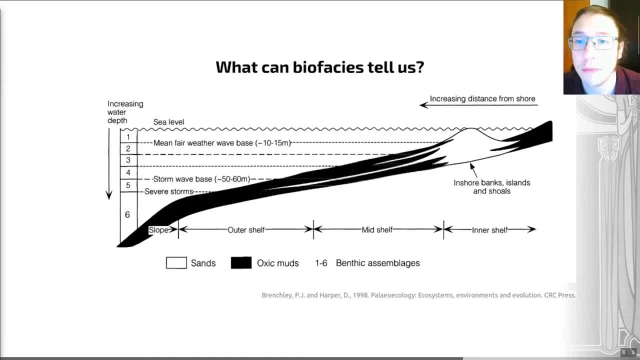 but also for those who are trying to understand patterns in past life. So, for example, sea level change and its changes. sorry, sea level change and its changes. no, the changes in sea level that we see in rocks help us understand the impact of climate fluctuations and then help us map the 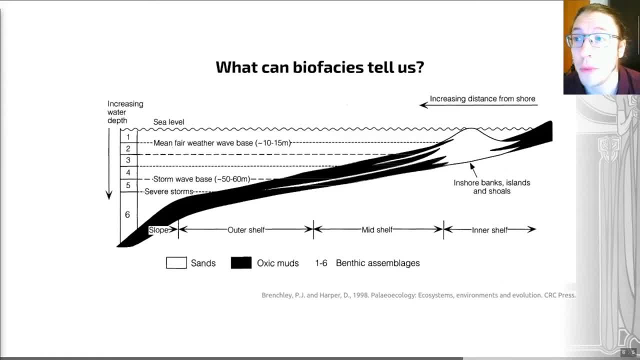 changes that we're seeing in sea level, and probably in climate, to responses in the biological community. Hence me including all of this here. I think it's really quite important, actually. So that's all for this video. I hope you enjoyed it and I'll see you in the next one. 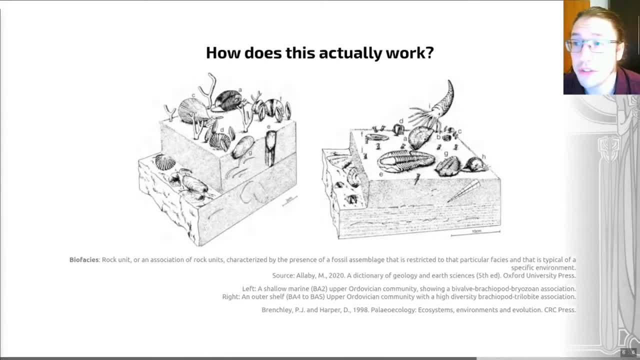 Bye for now. Thank you for watching. We can see an example of what we would find in deeper water. so somewhere around benthic, assemblage 4.. And in the upper order vision, this community had a high diversity of brachiopods and these were associated with trilobites. So what I'm trying to get at with. 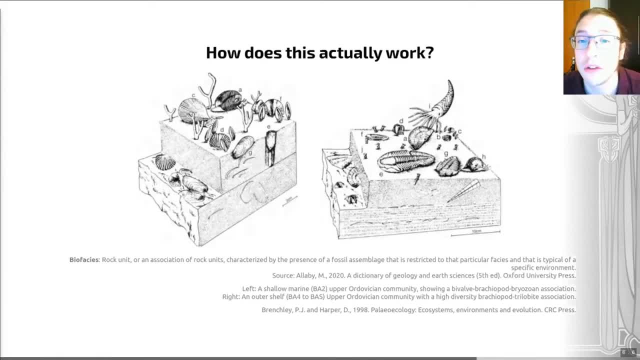 this slide and with the story of benthic assemblages, is that with a great deal of study, we can start to untangle changes in the environment and changes in environmental conditions in the fossil record from geography and from evolution. This can help us understand not only 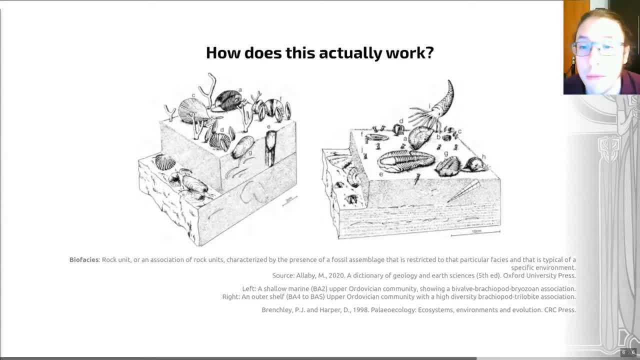 how environmental conditions change in deep time but how the groups that were alive at that time responded to it kind of writ large. I'm going to have more on this kind of like trying to understand the, the interplay of evolution and ecology on this really big scale in the more video. 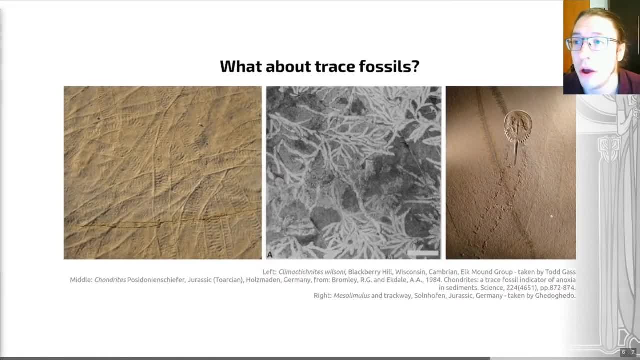 in the next video. I wanted to finish by highlighting trace fossils. So so far we've looked at body fossils, the remains of animals, but also we can consider the traces of animal behavior or fossilized sedimentary structures that were left by animals when they 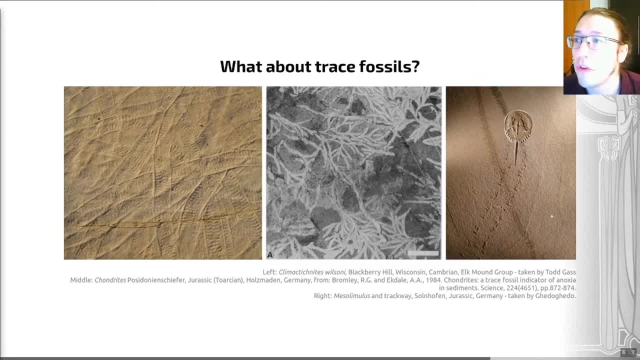 were alive. So body fossils will very rarely give you information about behavior and, in contrast, trace fossils are, by definition, the record of behavior of an animal when it was living, Be that locomotion as shown on the left hand side here, be that locomotion and feeding as shown in the middle here, or even the last. 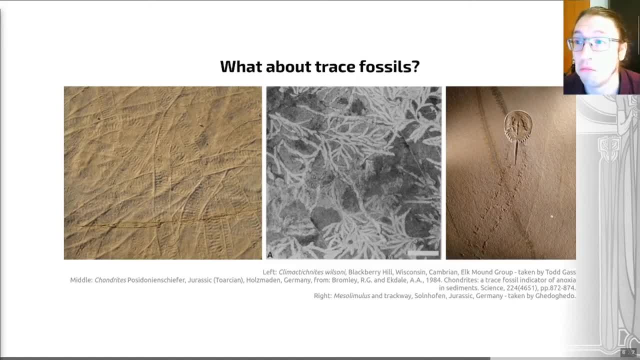 moments of an organism as it was walking towards its death. very metal And trace fossils are really important because of that, because they record behaviour, And behaviour is often environmentally controlled, And there's been extensive work done on using trace fossils, especially burrows, to determine the water depth at the point when that trace was made. 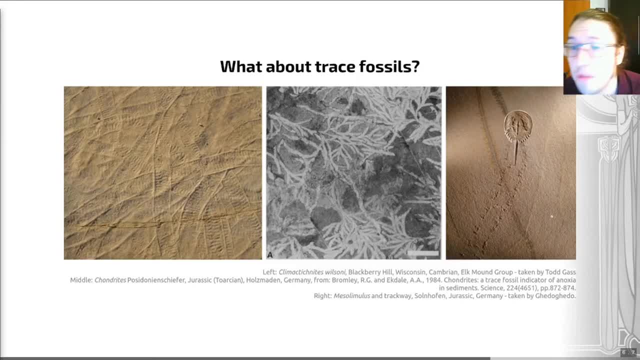 Some traces, such as the one on the far right here, can be relatively easily associated with a trace maker. In this case that's a horseshoe crab, a Xyphus uran, and the trail that you can see running up to it is clearly made by that individual, So we can identify the trace maker. 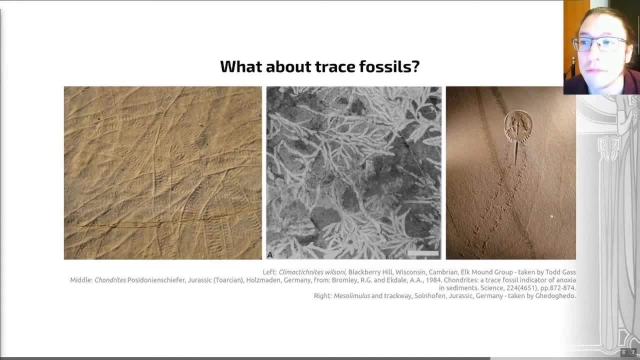 with its trace. But even when this isn't the case- and it isn't the case in many of the trace fossils that we want to look at- we can recognise distribution patterns. Just FYI: trace fossils get their own species name based on their shape. whether that's a good 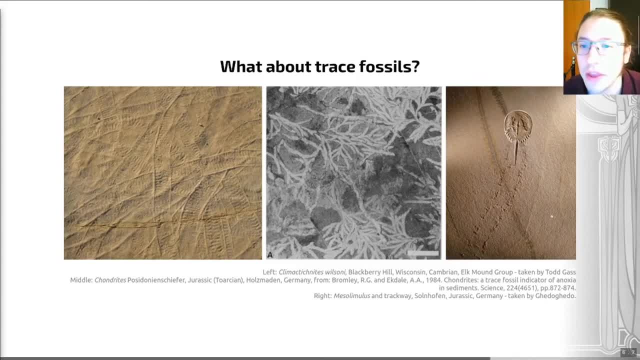 idea to do or not. I'm very happy to discuss. And they occur and we find them in both marine and terrestrial environments, but once more I'm going to focus on the marine environment. So when we're thinking about trace fossils, what we can do is we can identify onshore to offshore. 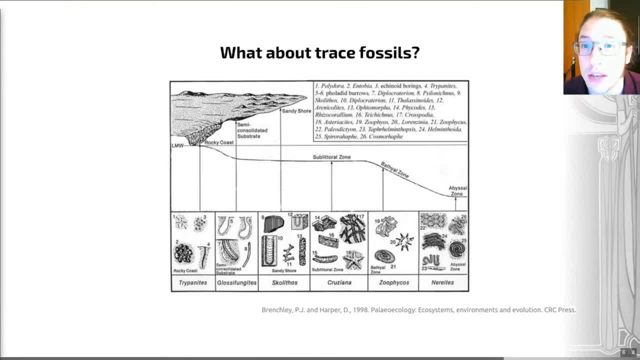 afections of the enviroment. So this is really interesting notice the little triangle here, as the stopped image, has mostly beenoderated into the past and once more the 마스�illes fit inside of them, gradients in the trace fossils that we see. And those gradients take us from intertidal 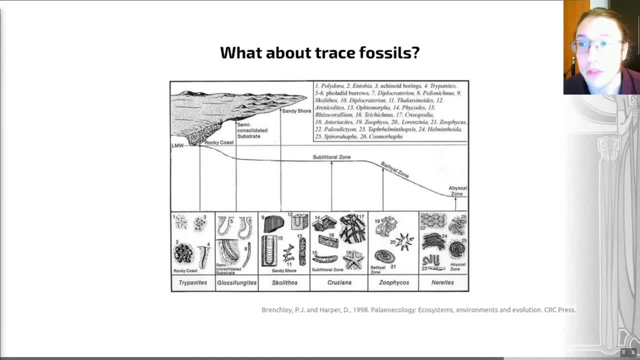 environments all the way through to the deep sea. The same as we had biofaces, we can organize these trace fossils into categories that we call ignofaces, each developed on and within soft, unconsolidated sediments. So we need to have soft sediments for these to work. but they can tell us. 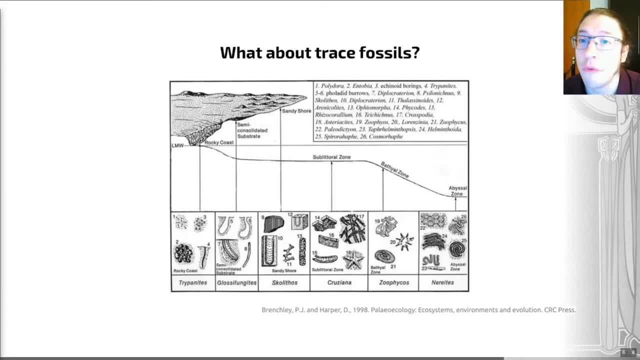 something about the depth of water And there are four main ignofaces which we associate with depth. So these are the Skelethos faces, the Cruciana faces, the Zooficos faces and the Nereides faces, These four here. I don't think you need to know much more about them than that, because for the 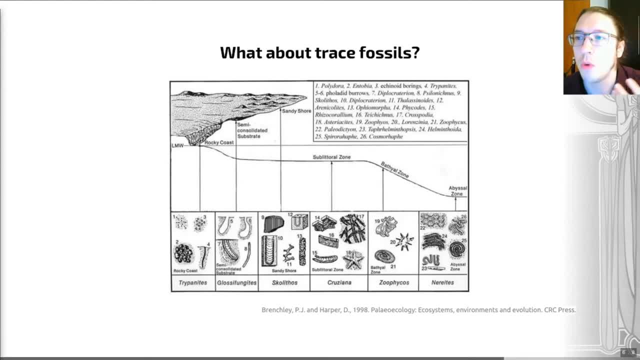 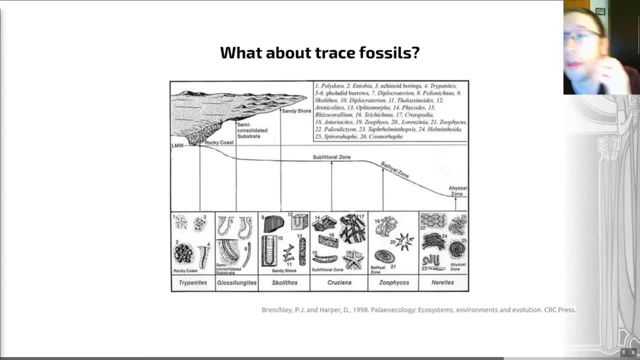 they can take a look at the depth of water and how they can use both fossils and trace fossils to tell water depth, And knowing that these ignofaces exist is easily enough for our needs for this course. I should highlight that the general trends I've talked about have been criticized. 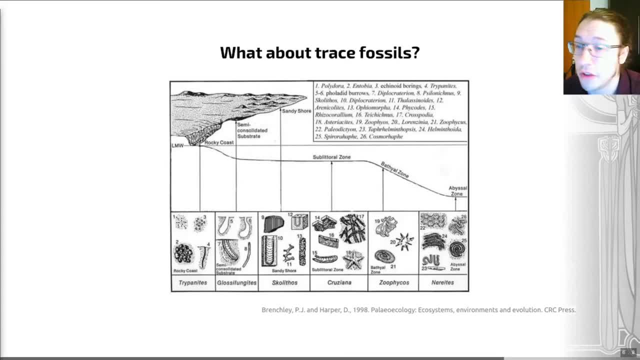 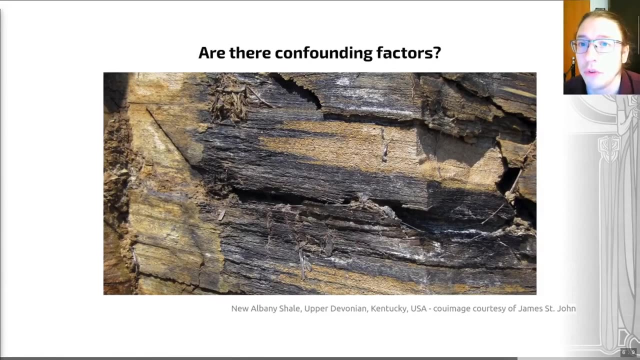 because sometimes the behaviors that these trace fossils record are influenced by both turbulence of water, the rate of sedimentation, the availability of food and the oxygen concentration in an environment. So bear in mind that this is all a very nuanced picture And fossils can be used. 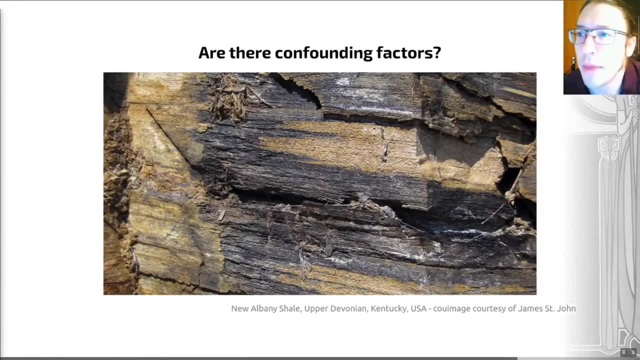 used as indicators for other conditions which again may interest us greatly if we're looking at evolution in the deep past and the evolution of the earth life system in the deep past. so, for example, in oxygen poor environments we expect darker carbon rich sediments. those will have decreased biotubation, so decreased burrowing, and that will often be marked by the preservation. 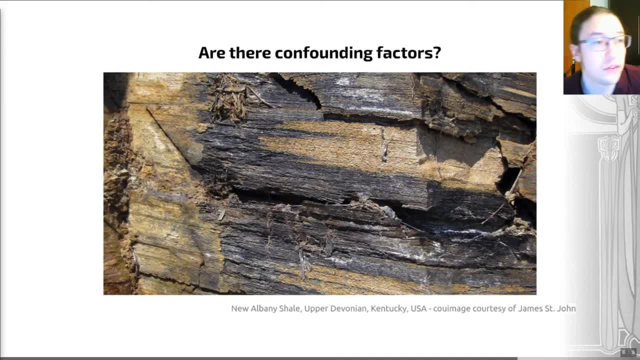 of delicate sedimentary layers, such as shown in this dark shale in the upper devonian of the kentucky in the usa. here we'll often see particular trace fossils. there's a famous one called chondrites, which is associated with low oxygen environments. in these low oxygen, 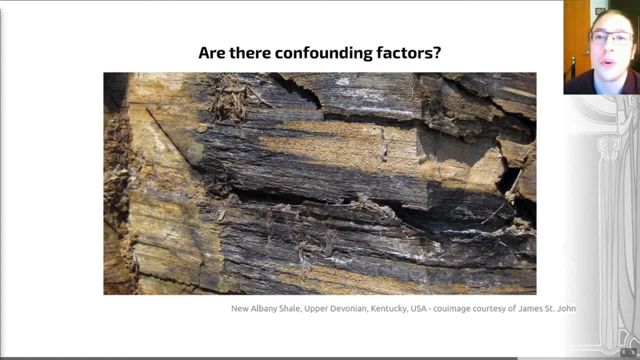 environments, benthic fauna, so the fossils show a decline in species diversity. there's also a decrease in size and in the depth of burrows- where you do have burrows. so essentially what we're looking at is that we're we when we're looking at a rock we have. 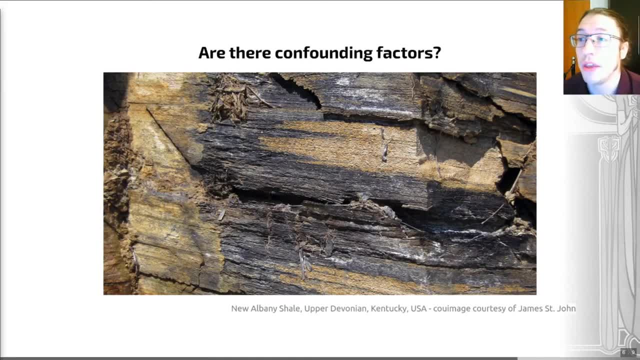 a mix of factors that impact on the sedimentary record and the fossil record that we see in those rocks. these can be really useful to help us understand what's going on in earth history and in life history, but we have to study each individual rock as a unit in and of itself.